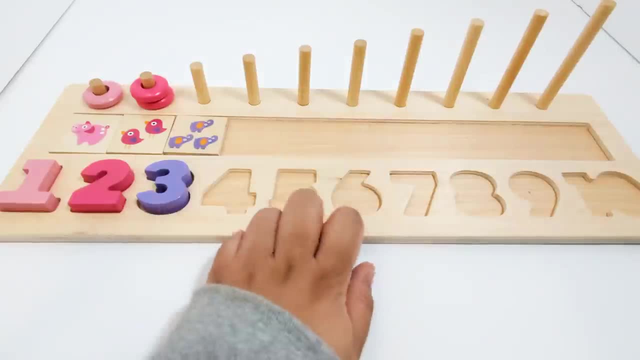 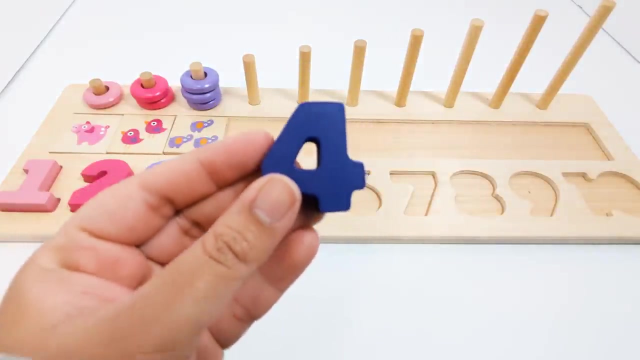 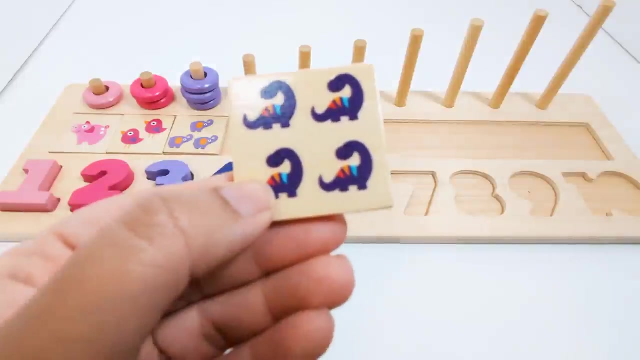 Three light purple or lilac pieces: One, two, three. One, two and three. Now which number comes after the number three? That's right, It's the number four. This number four is purple. This piece has four dinosaurs on it. 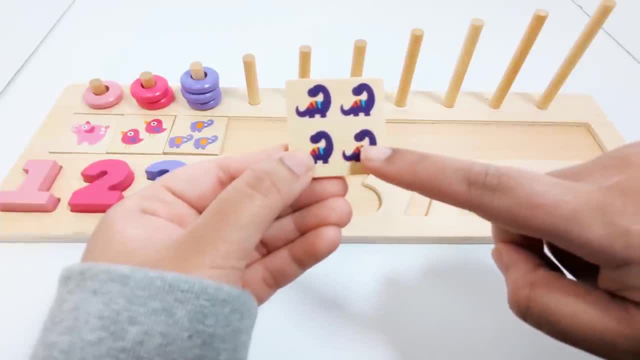 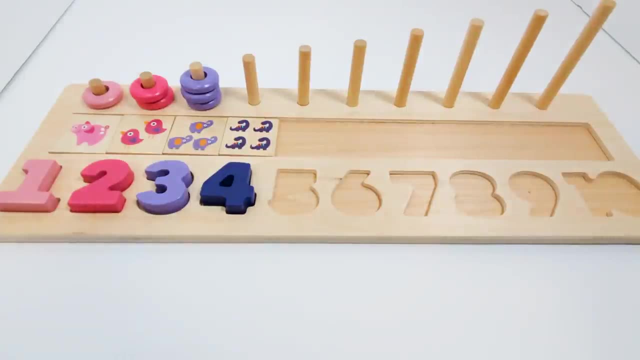 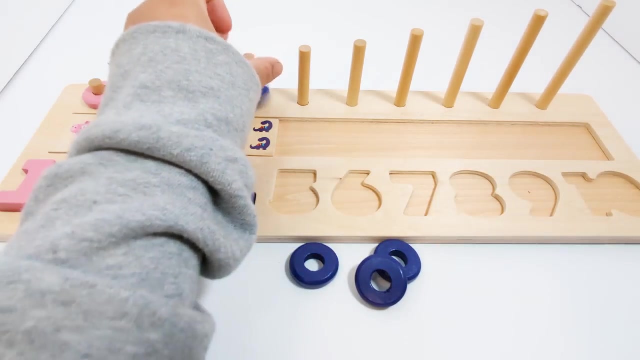 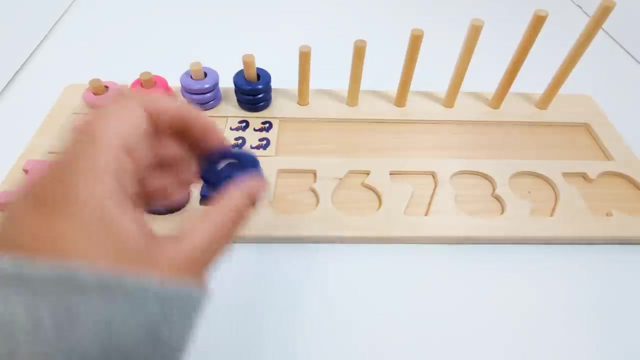 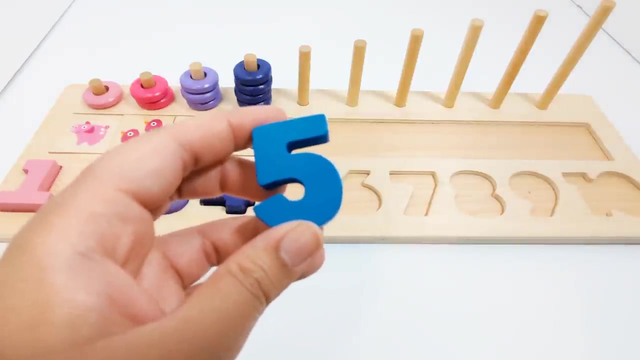 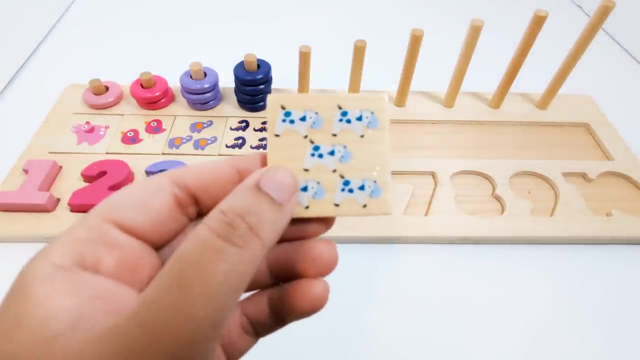 One, two, three, four, Four purple dinosaurs, Four purple pieces: One, two, three and four. Which number comes after the number four? That's right, The number five. This number five is the color blue. There are five cows on this piece. 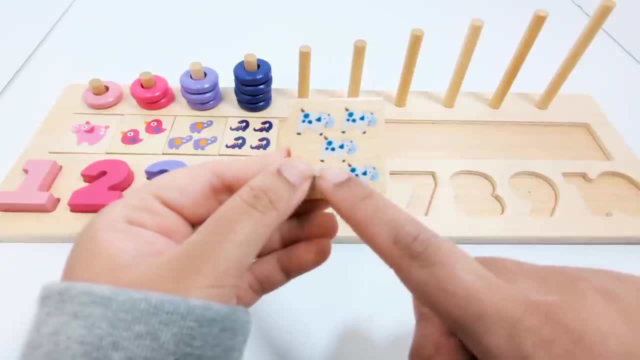 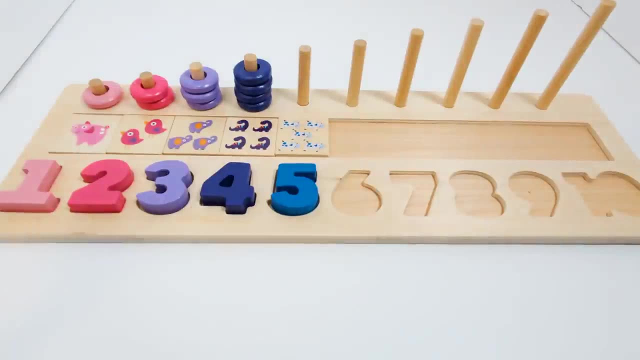 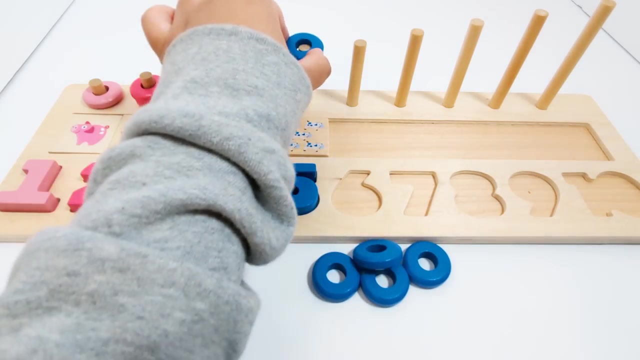 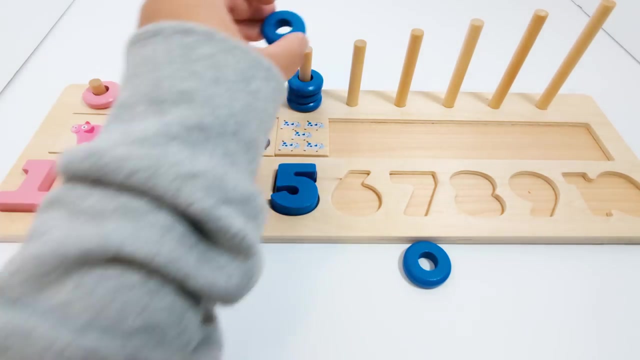 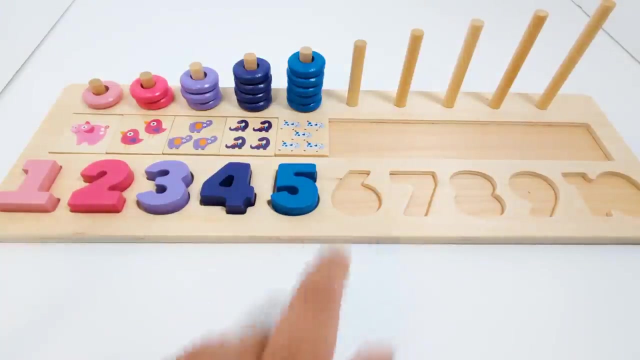 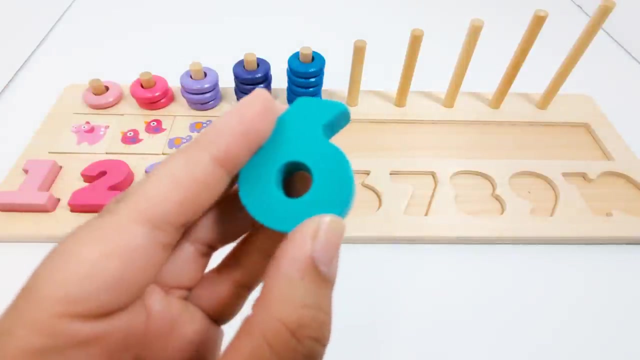 One, two, three, four, five, Five cows, Five blue pieces. Five blue pieces: One, two, three, four, five. Which number comes after the number five? That's right, The number six. This number six is turquoise. 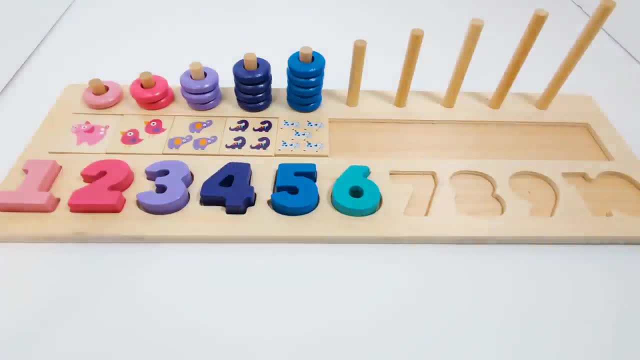 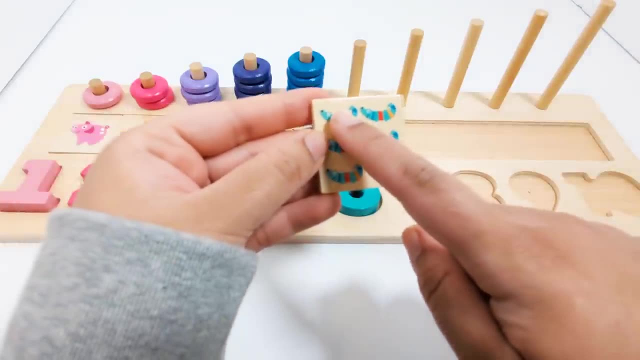 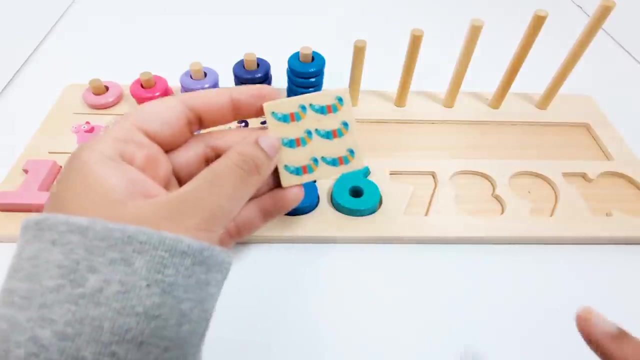 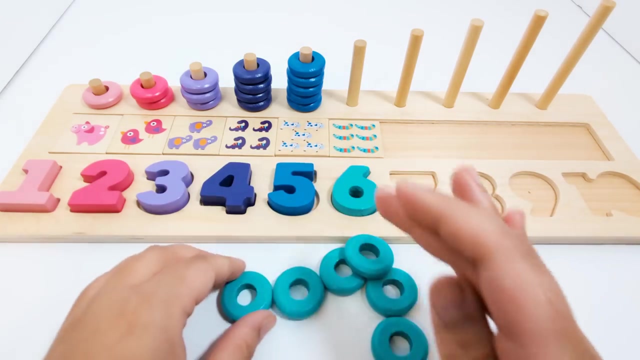 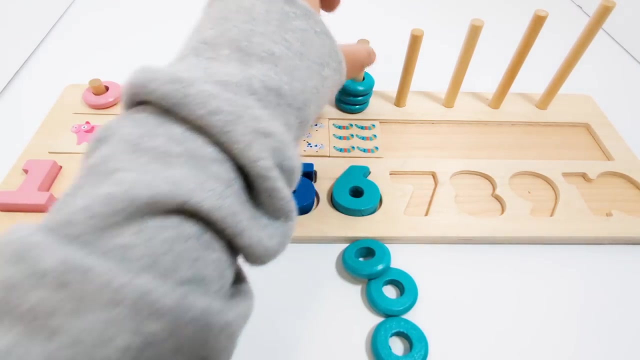 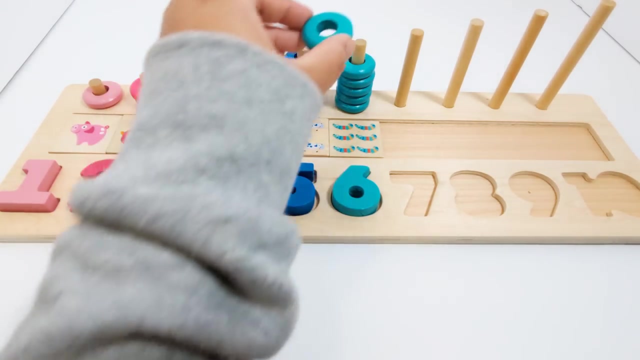 This number six is turquoise. There are six crocodiles on this piece: One, two, three, four, five, six. Six turquoise pieces: One, two, three, four, five. Two, three, four, five and six. 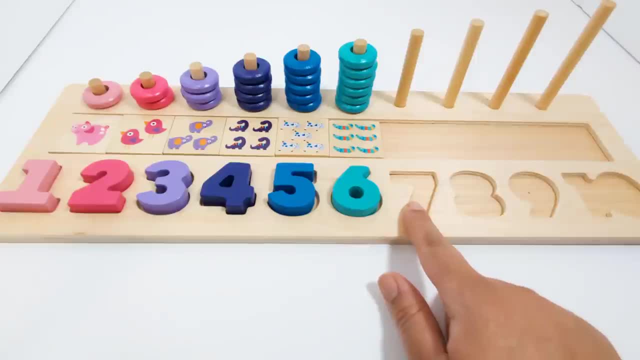 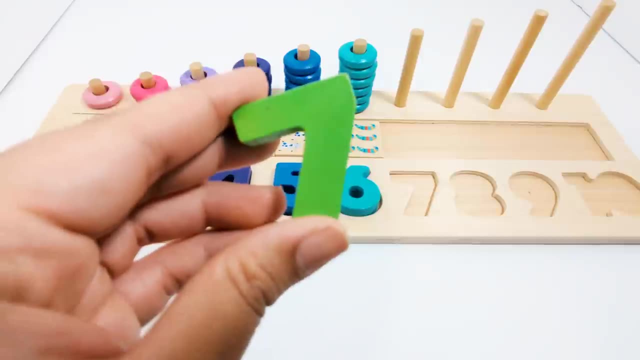 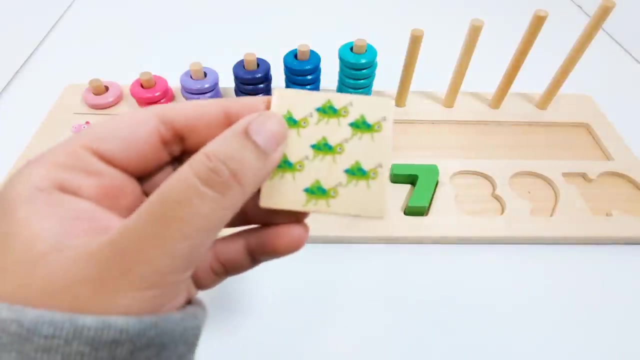 One, two, three, four, five and six. Two, three, four, five and six. Who's number comes after the number six? That's right, The number seven. This number seven is green. There are seven grasshoppers on this piece. 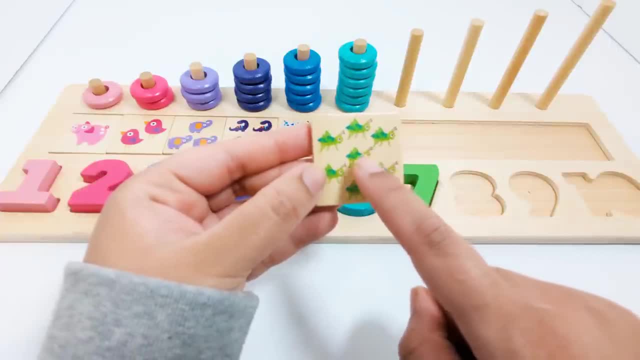 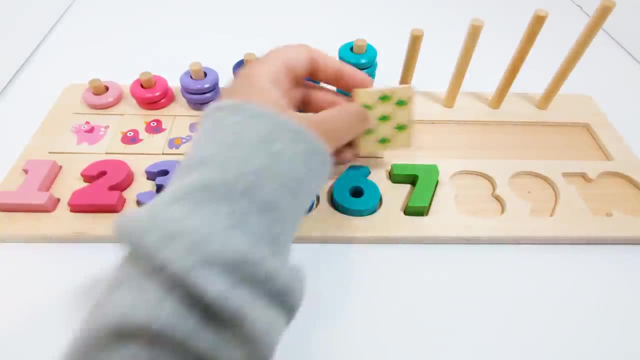 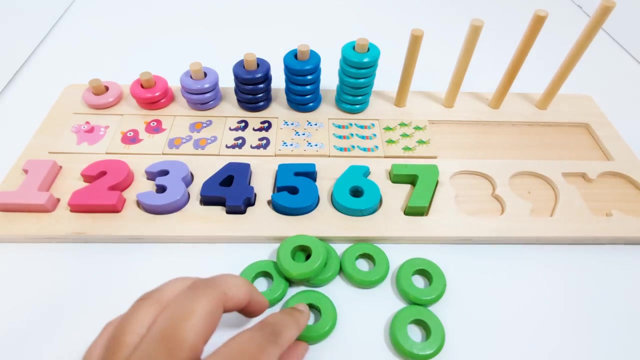 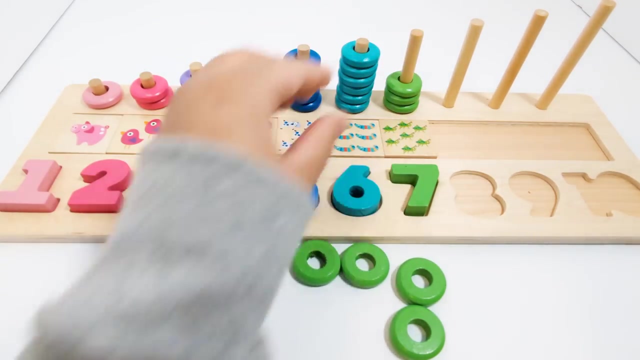 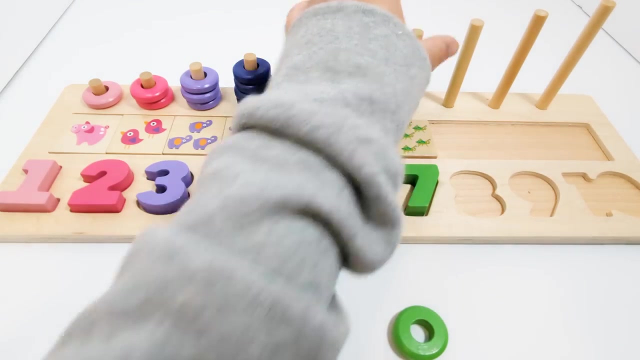 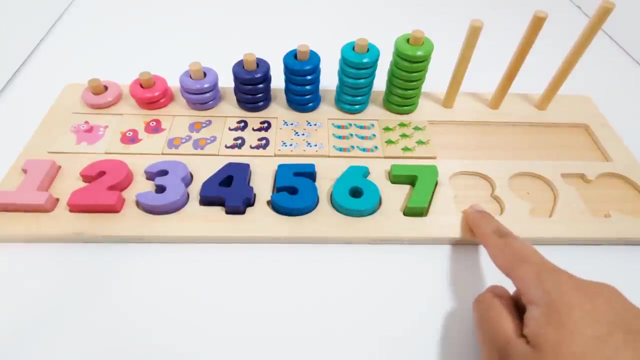 One, two, three, four, five, six, seven, Seven grasshoppers, Seven green pieces: One, two, three, four, five, six, seven. Which number comes after the number seven? That's right, the number eight. 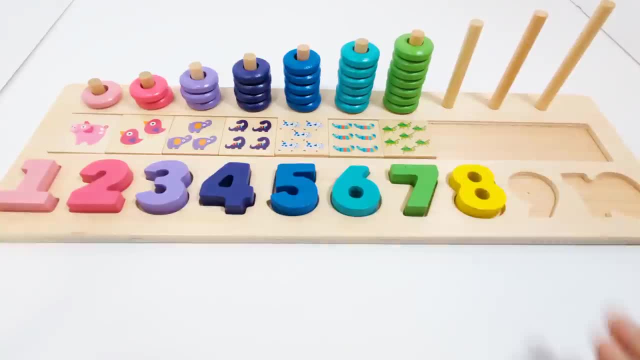 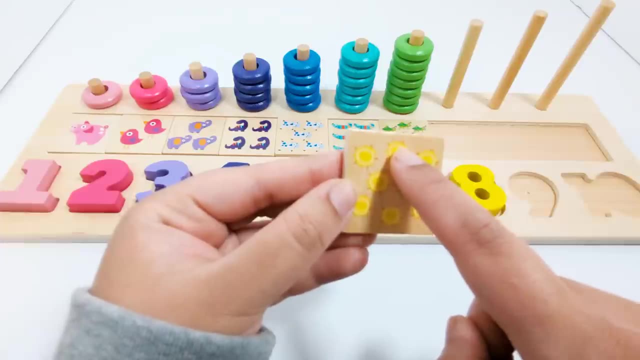 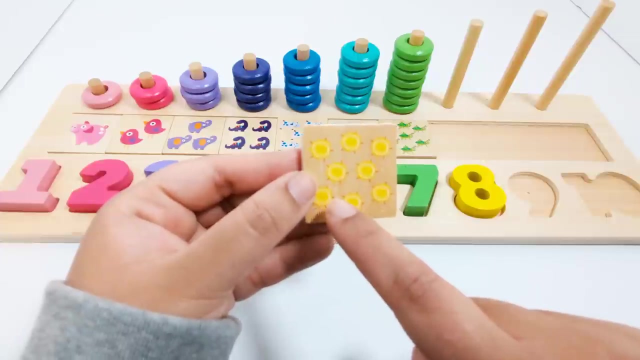 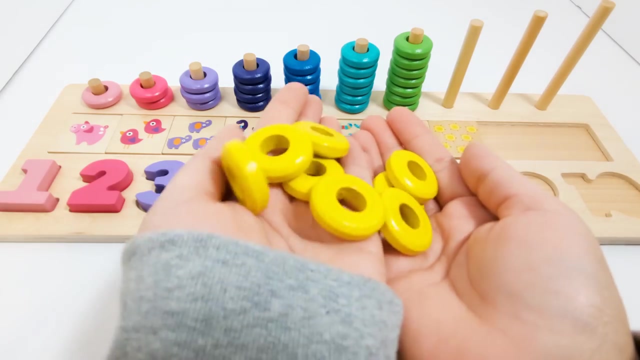 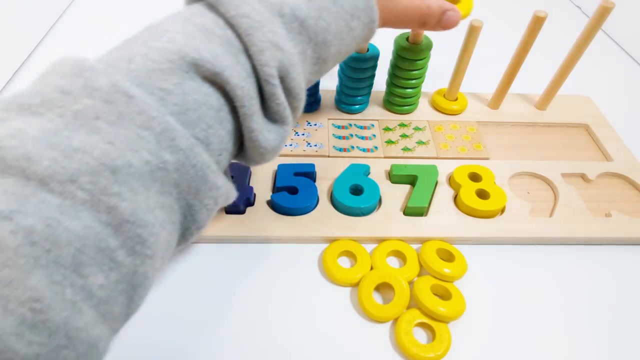 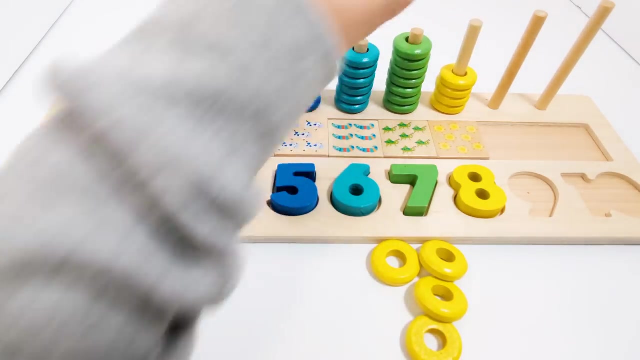 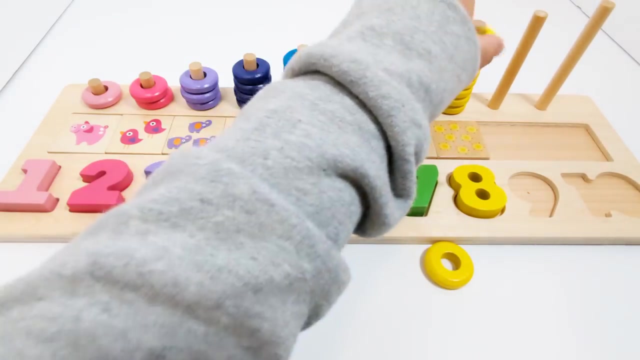 This number eight is yellow. There are eight suns on this piece: One, two, three, four, five, six, seven, eight. Eight yellow pieces: One, two, three, four, five, six, seven and eight. 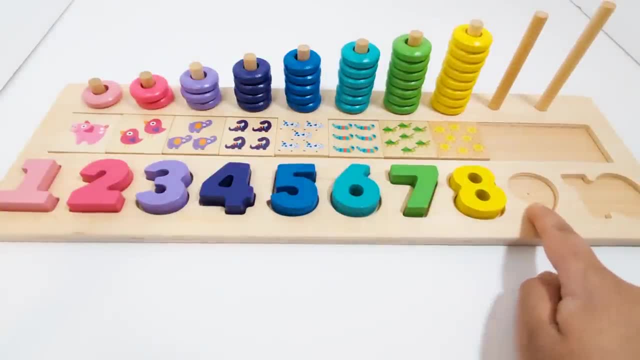 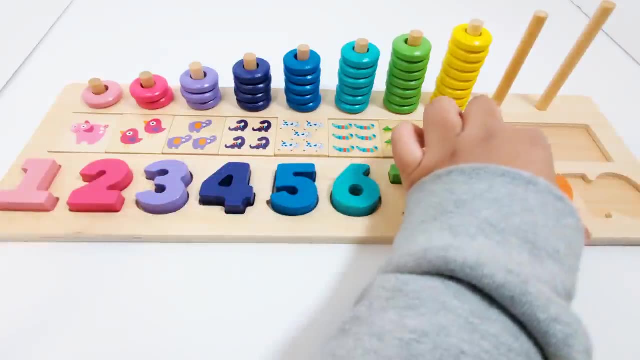 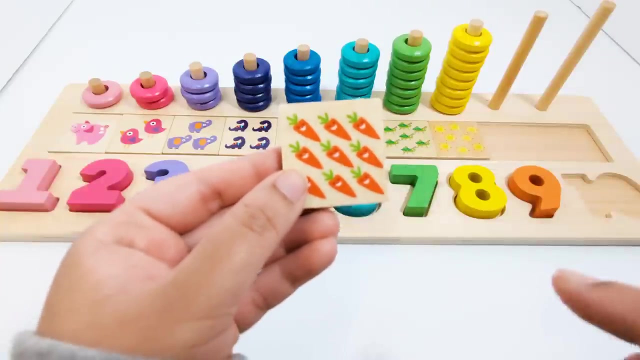 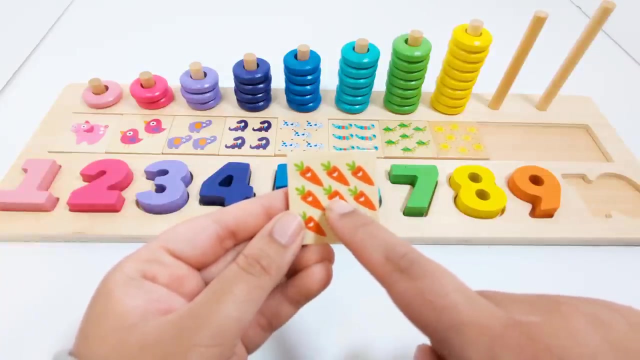 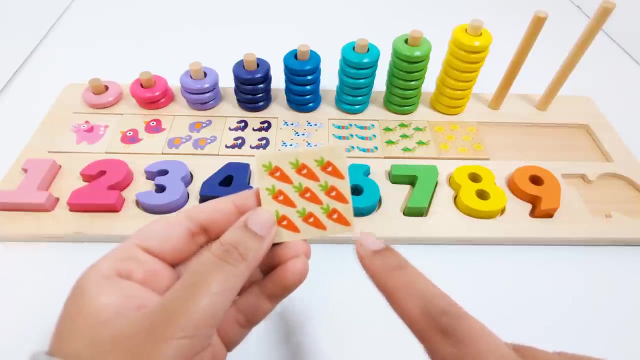 Which number comes after? the number eight? That's right. the number nine. This number nine is orange. That's right. the number nine is yellow, That's right. the number nine is orange. There are nine carrots on this piece: One, two, three, four, five, six, seven, eight, nine.